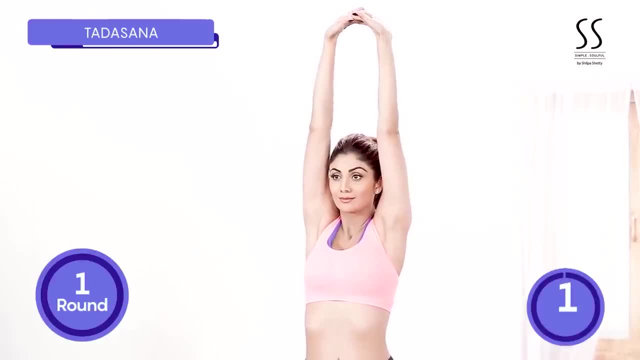 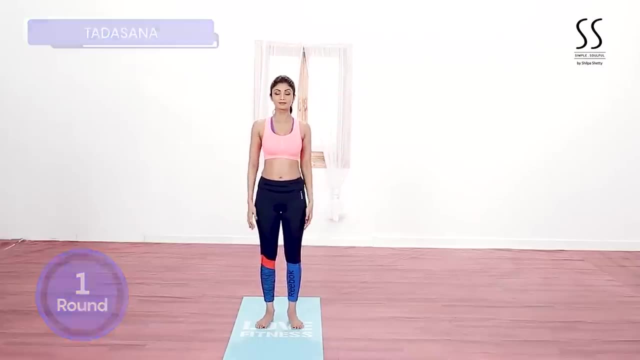 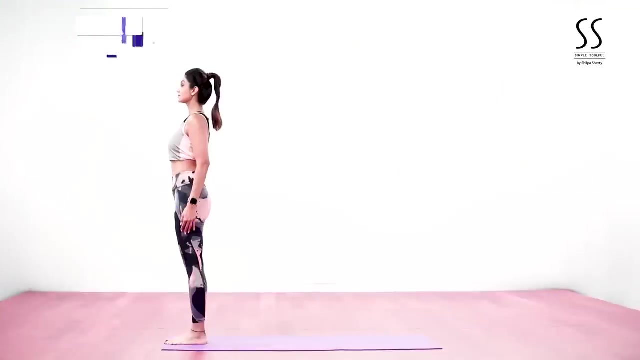 Maintain normal breathing pace. Come back to the starting position. The next exercise is called Prakashana. Stand erect at the top edge of the mat with your feet together. Bring your palms together in front of your chest. in Pranamasana, Inhale, raise your arms to the ceiling and arch your back as per your flexibility and come into Hastaruttanasana. 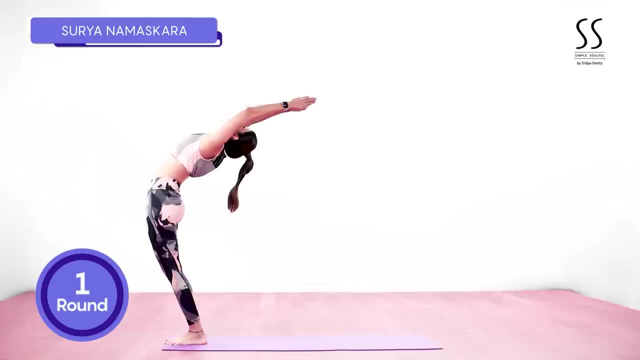 Exhale. bend forward from your waist, keeping your back flat. Bring your palms down on the floor and rest your back on the floor. Maintain weight at the top edge of the mat. Maintain your hands in front of your chest. Maintain your arms in front of your chest. 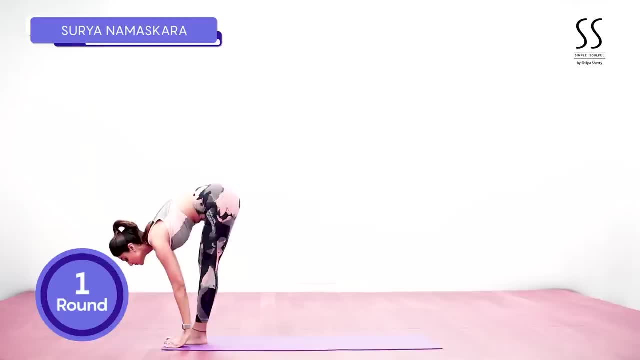 Maintain your arms in front of your chest floor, next to your feet in Padahastasana. Inhale, take your right foot backward, lower the hip and pull your shoulders back, Open your chest and look up in Ashwa Sanchalanasana. 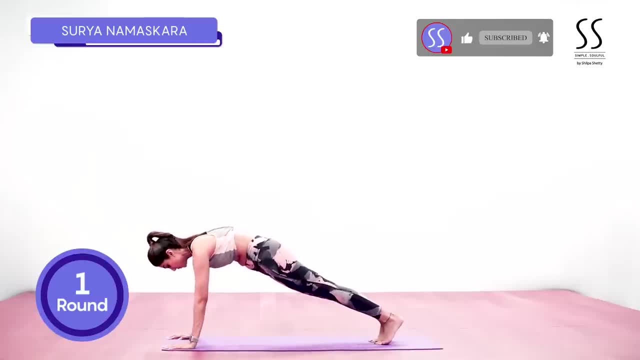 Exhale. take your left foot backward and come into the Udhit Chaturanga Dandasana. Make sure your shoulders are above the wrist and your entire body in slant position. Hold your breath and come into Ashtang Namaskarasana. Gently bring both your knees, your chest and 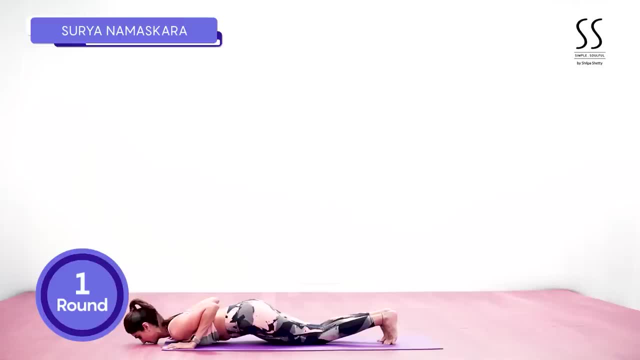 chin down on the floor while keeping your hip above the floor. Place your palms next to the chest and hands closer to the torso. Inhale, scoop forward and bring your chest upwards and forward and come into Bhujangasana. Now exhale, come into Parvatasana. Use the 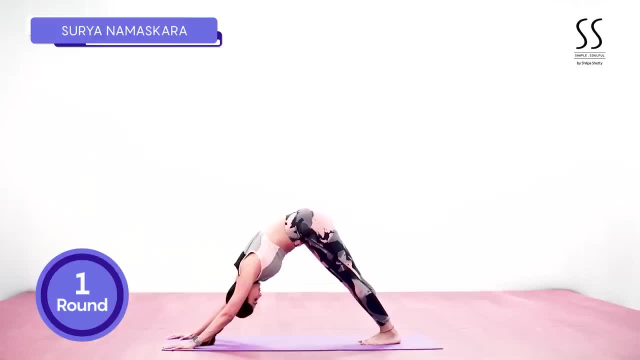 core to lift your hips up. Tuck your chin in towards the chest. Inhale. come into the Ashwa Sanchalanasana. Bring your right leg forward in between the hands. Lower the hips and look up. Exhale. bring your left foot forward and try to touch. 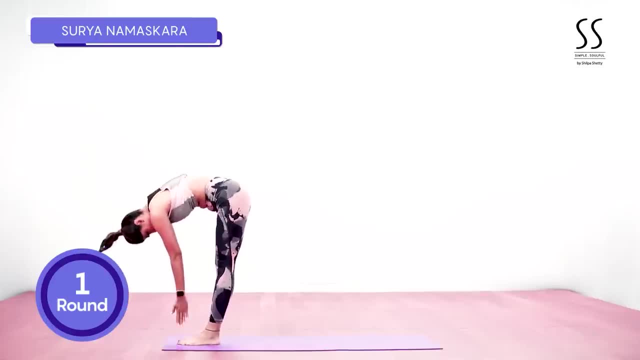 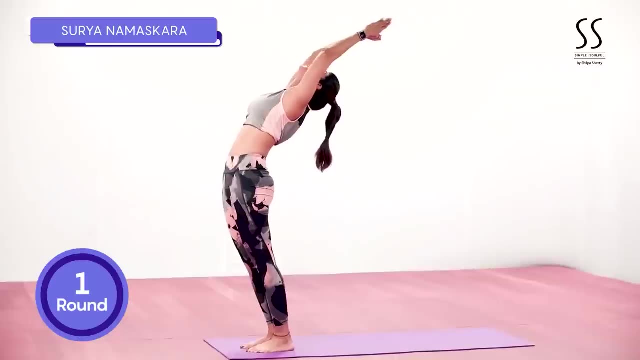 your palms on the floor in Padahastasana Inhale. lift your arms up, lengthen the spine, arch your back and come into Hasta Uttanasana Exhale. bring your palms together in front of your chest. 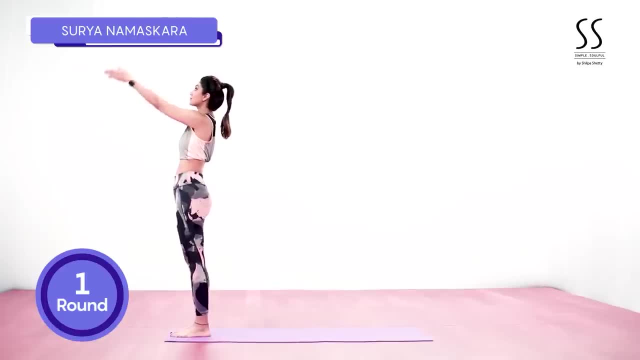 In Pranamasana, repeat the same steps with your other leg, and that will complete one cycle. Are all the movements working? Now it's time to forty-fourhimeni, Chapter Three Of the Ashwa Sanchalsana monter dana. 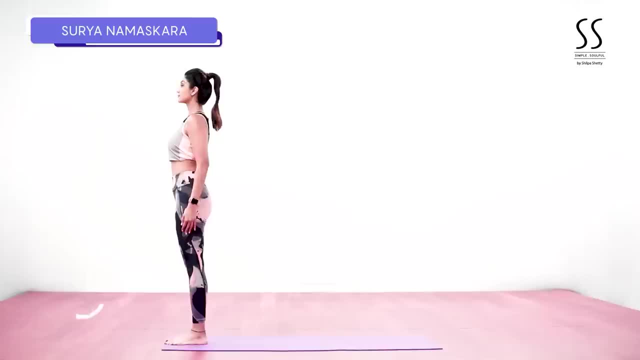 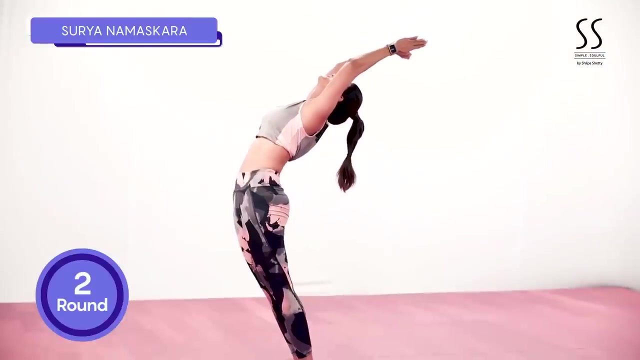 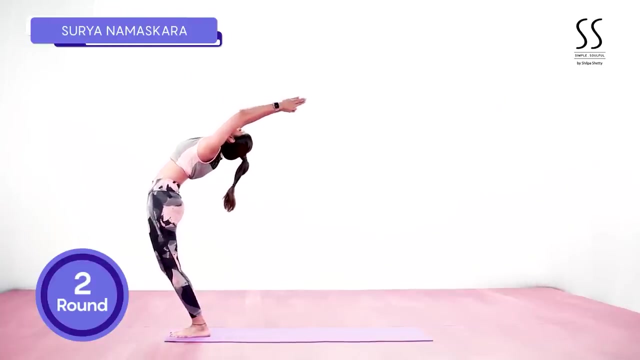 Asana Sanchalasana. Keep head in between arms and avoid tilting your head back too much. Keep your head in between arms and avoid tilting your head back too much. Keep your head in between arms and avoid tilting your head back too much. 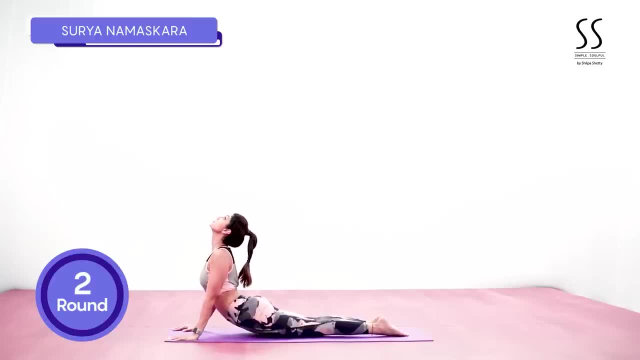 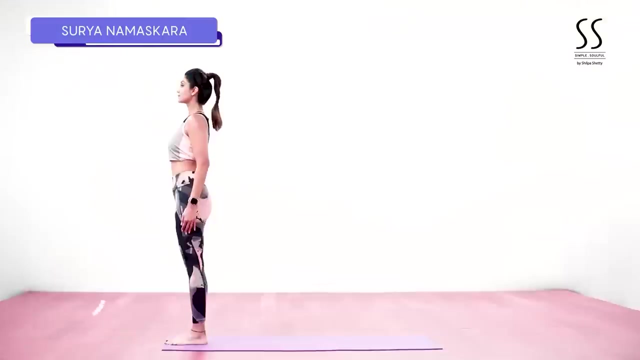 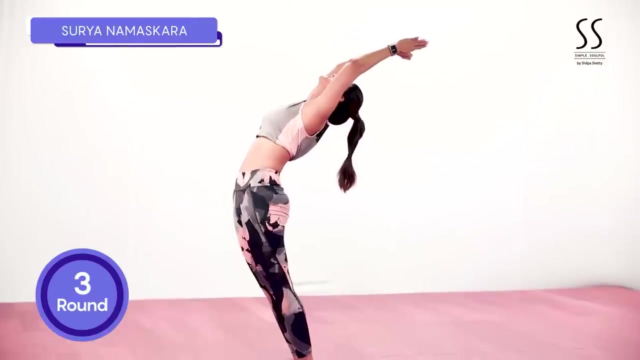 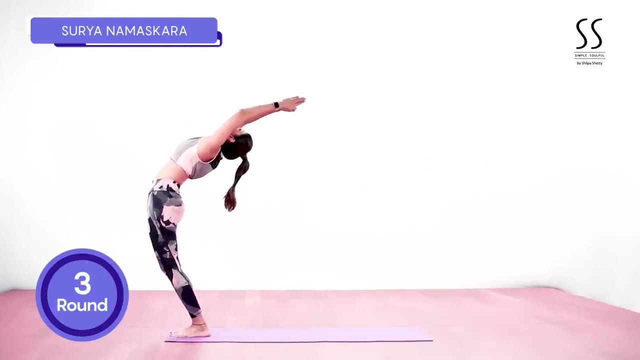 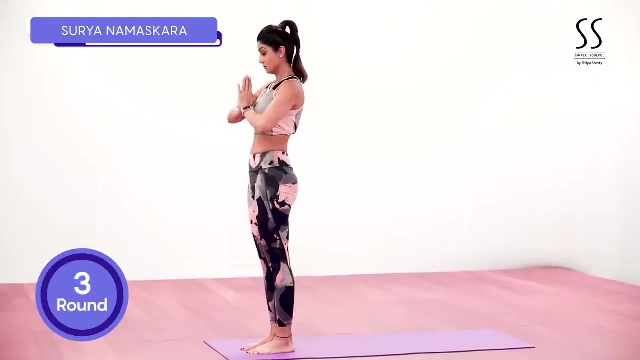 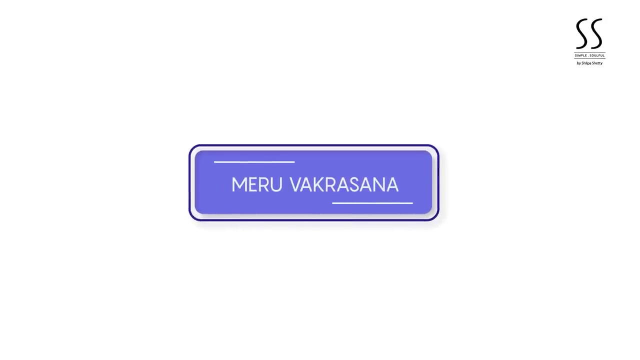 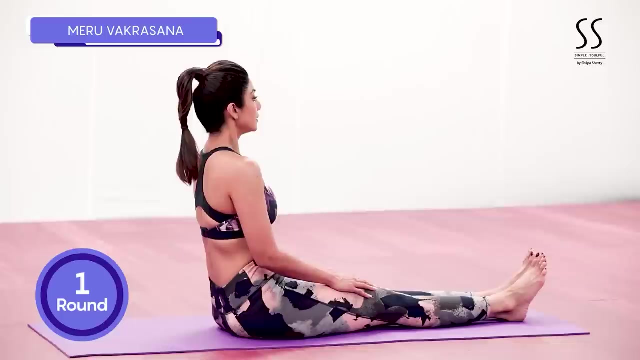 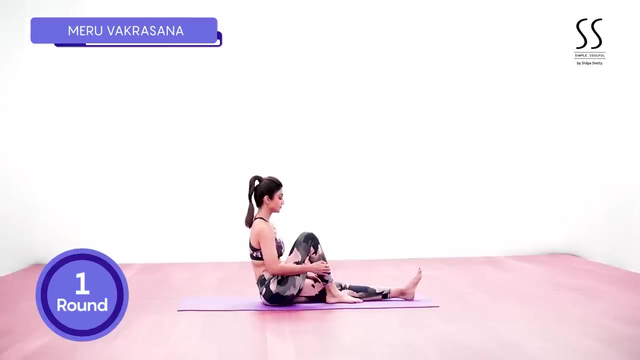 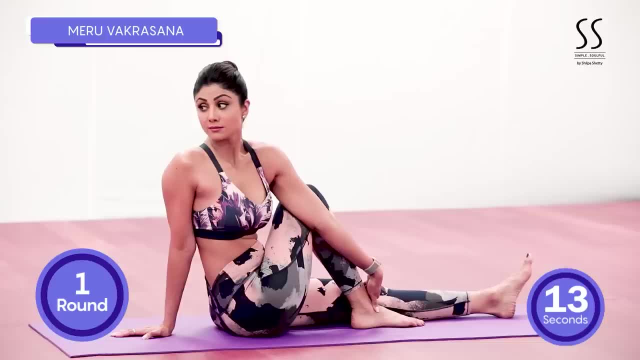 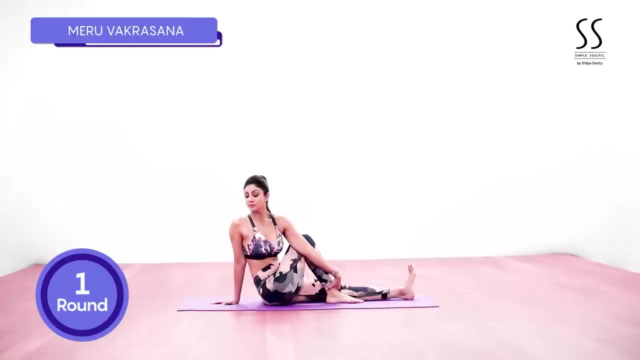 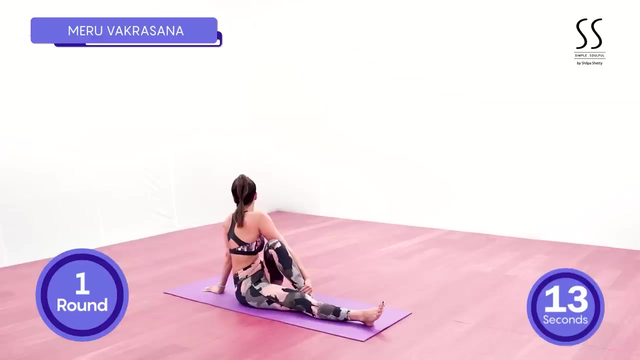 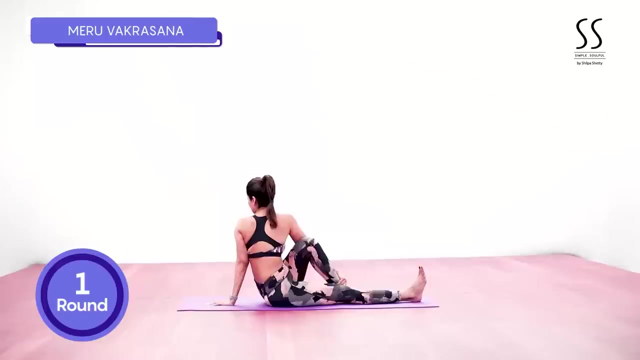 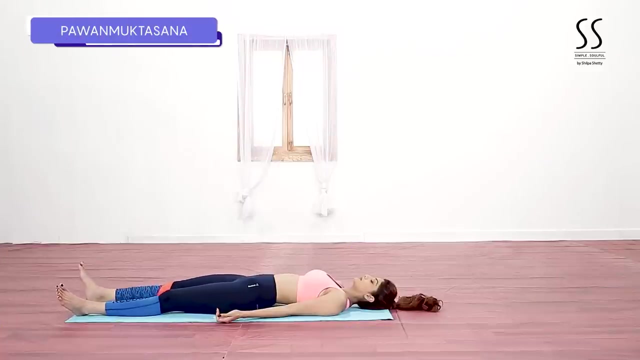 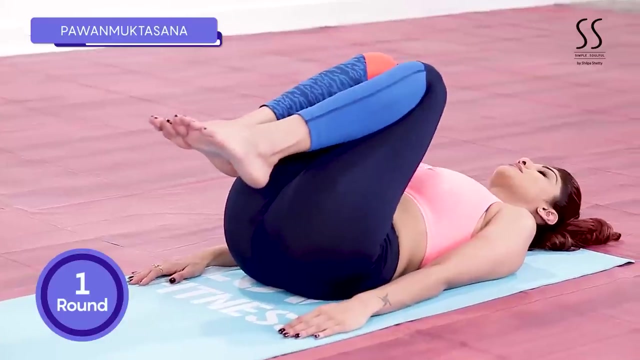 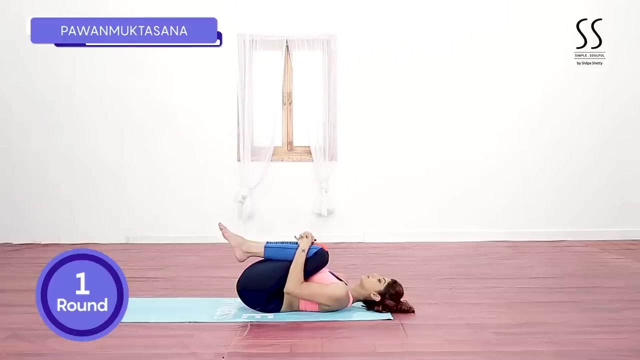 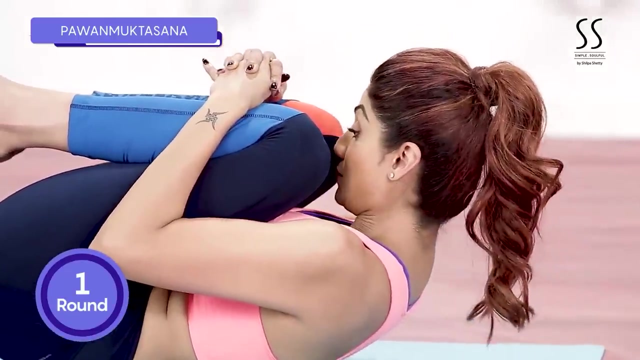 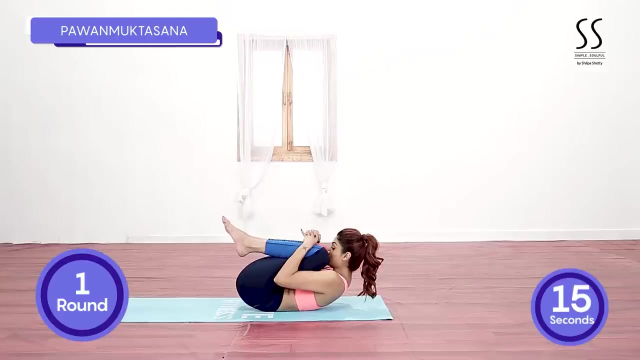 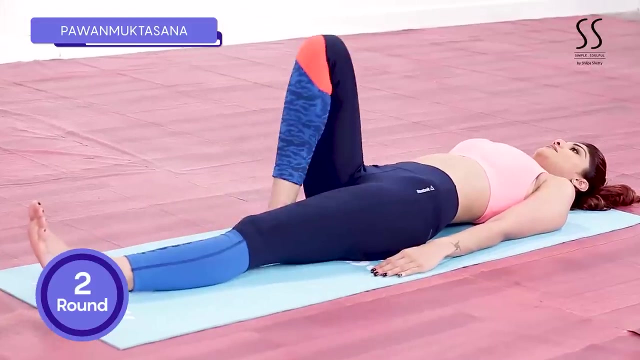 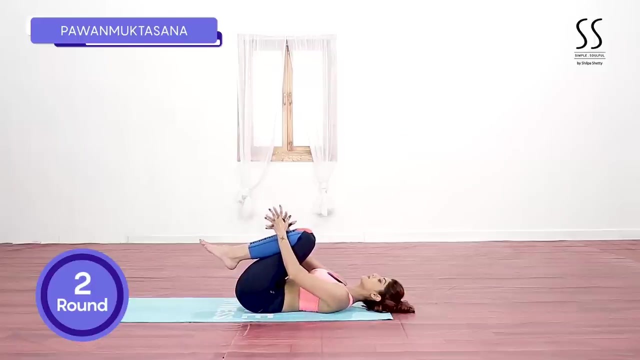 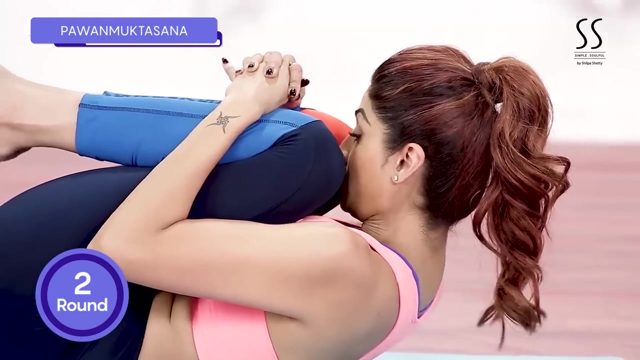 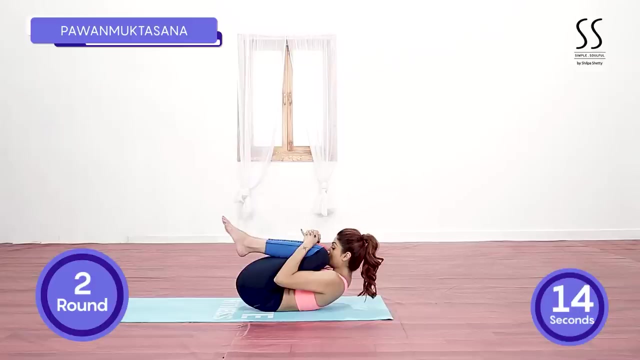 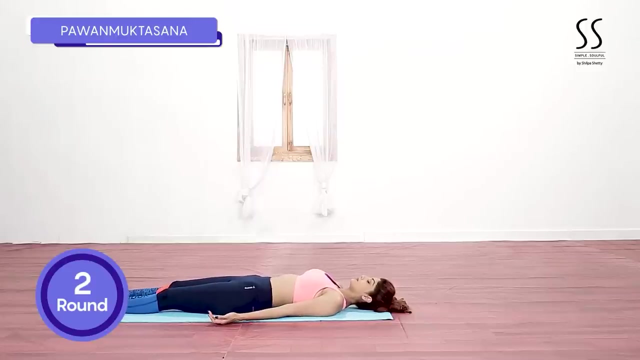 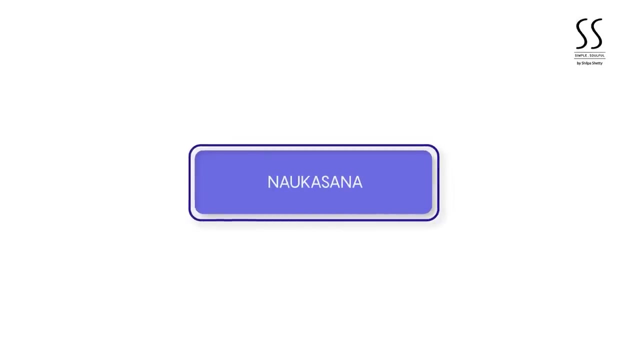 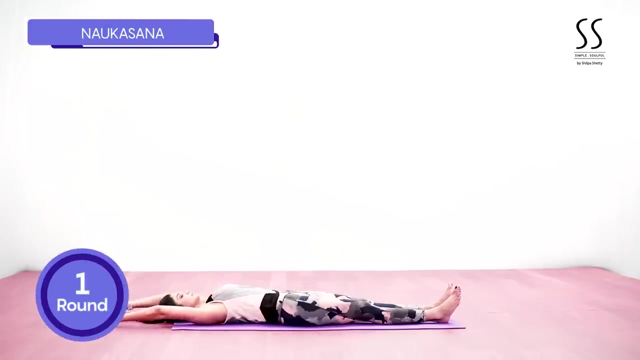 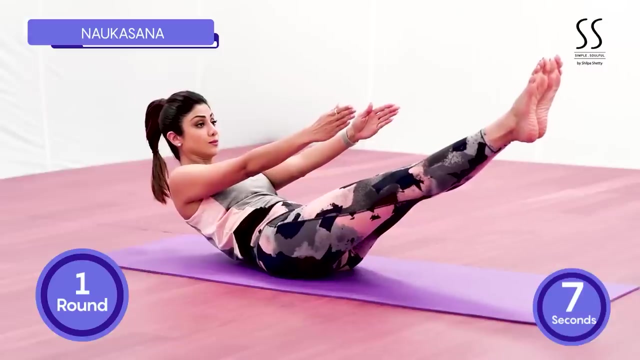 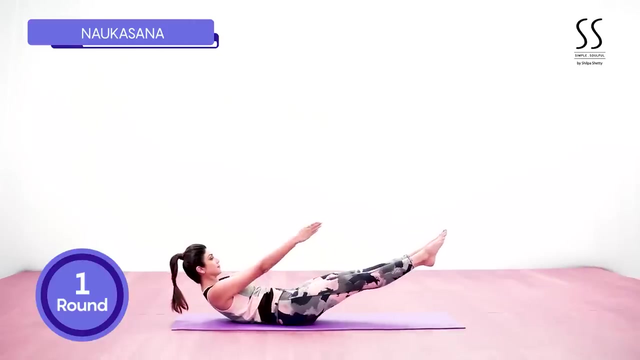 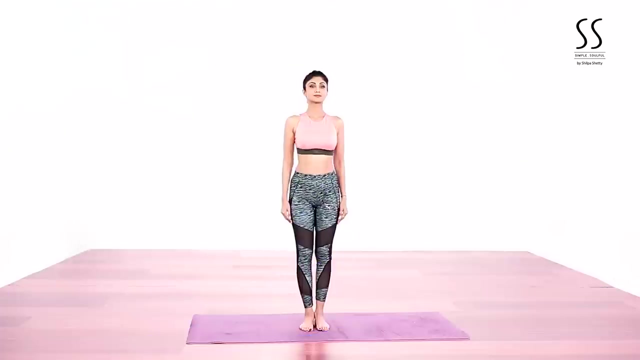 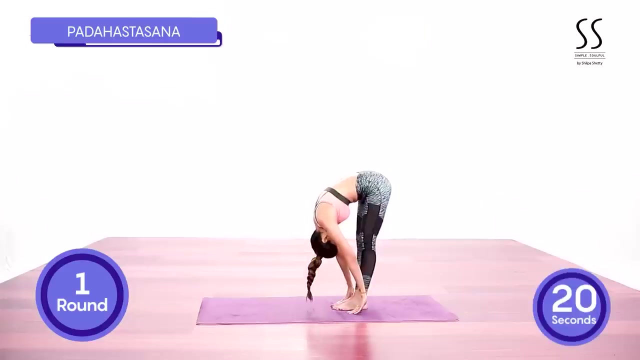 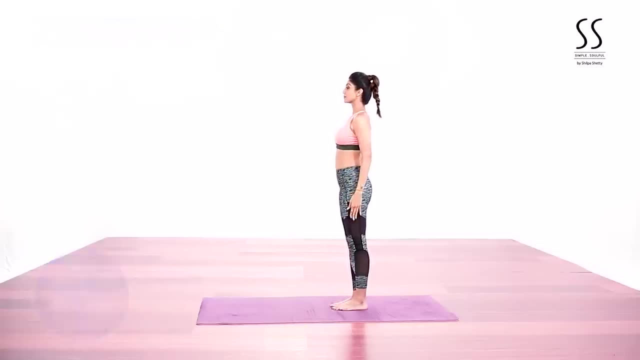 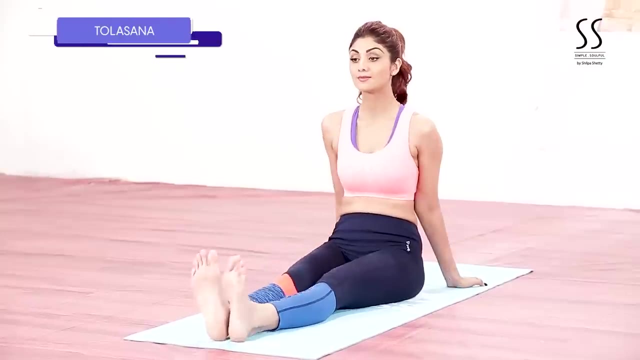 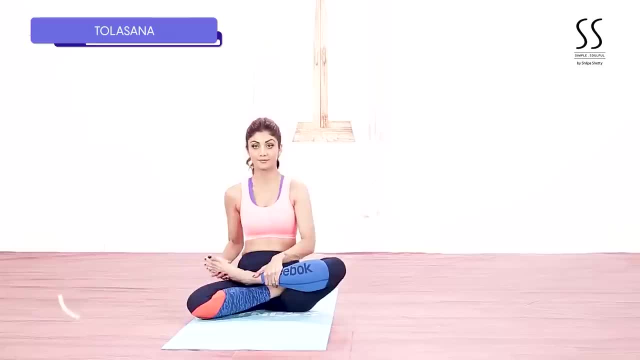 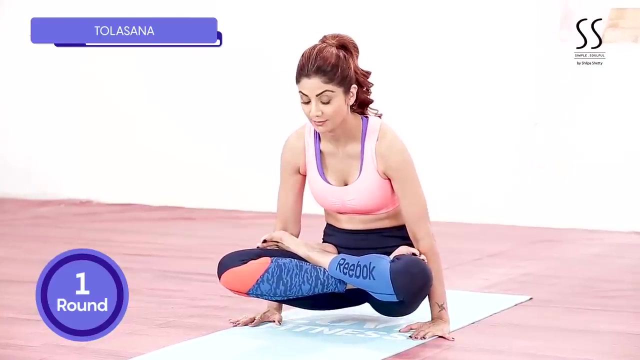 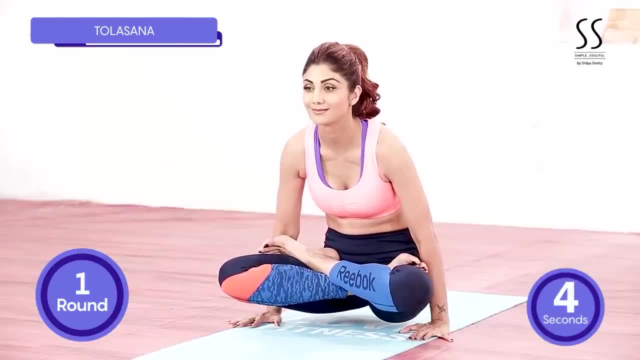 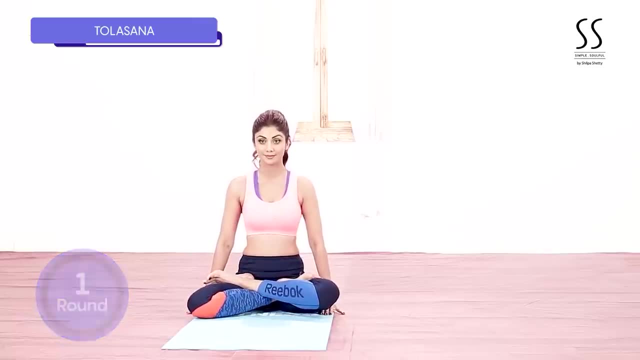 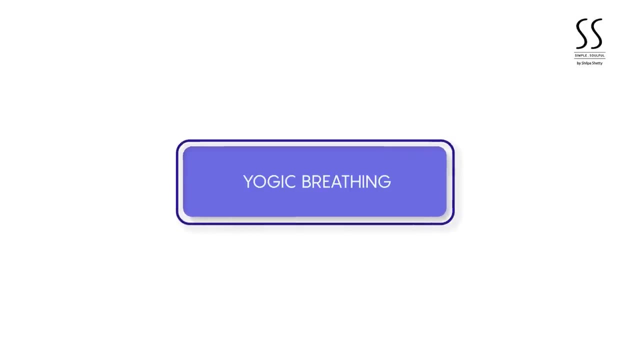 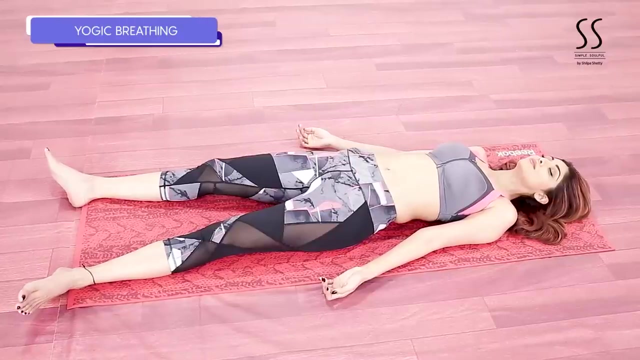 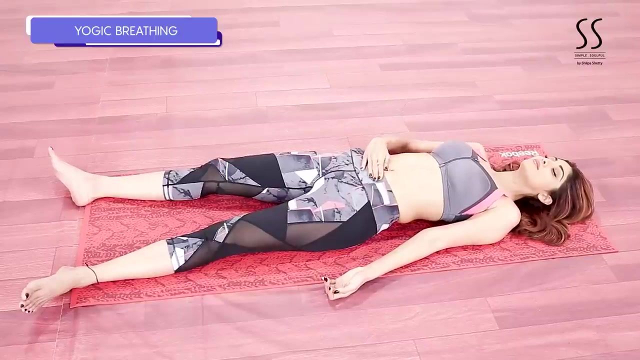 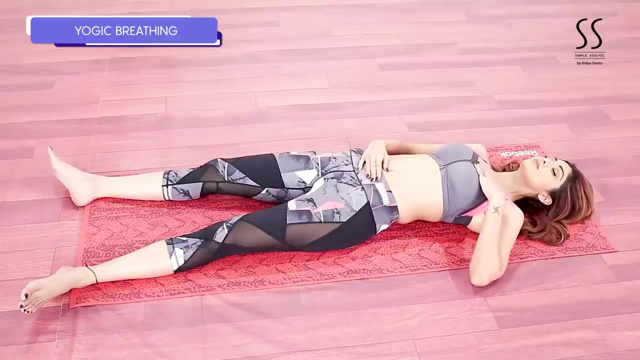 of pulling the legs towards the chest to engage your core. breathe only through the nose during this pose. then lower your hips, release your hands, come back to the starting position and relax. lie on your back with the legs apart and relax the whole body. place your right hand slightly below your navel and left hand on your left chest. inhale slowly. 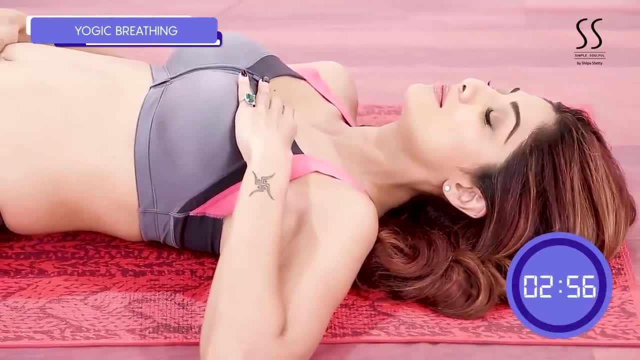 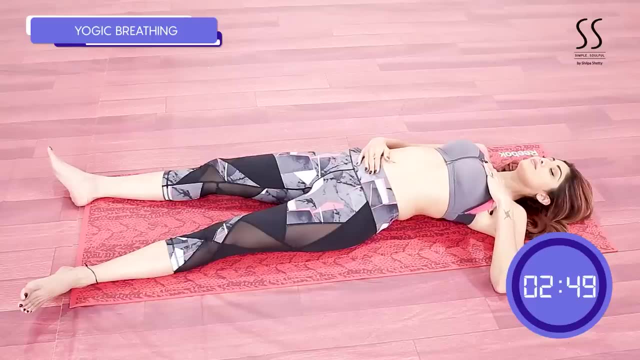 and exhale and deeply fill the belly up with your breath. expand the belly with air like a balloon. when the belly is full, draw in a little more breath and let that air expand into the ribcage. let it fill the upper chest all the way up to the 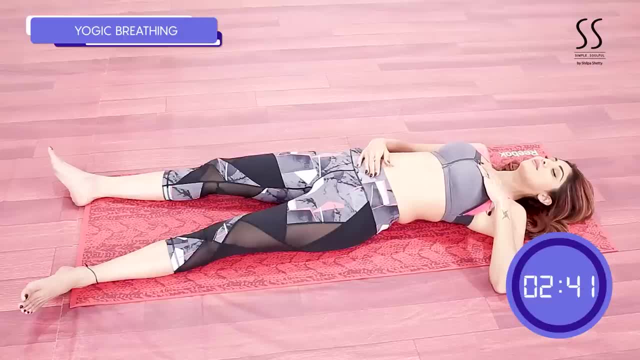 collarbone on the exhale. let the breath go first from the upper chest, allowing the heart center to sink back down, then from the ribcage, letting the ribs slide closer together. finally, let the air go from the belly, drawing the navel back towards the spine. this is one yogic. 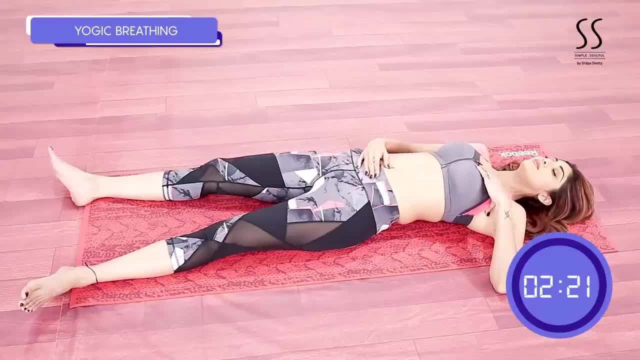 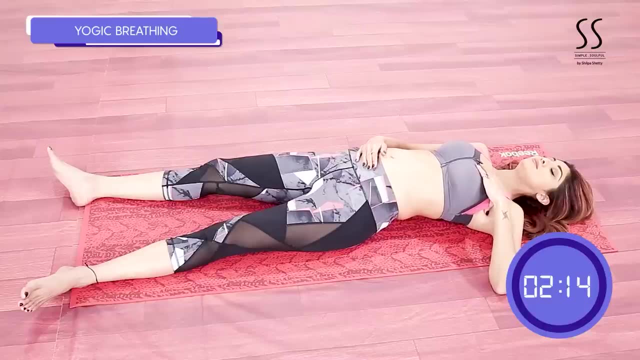 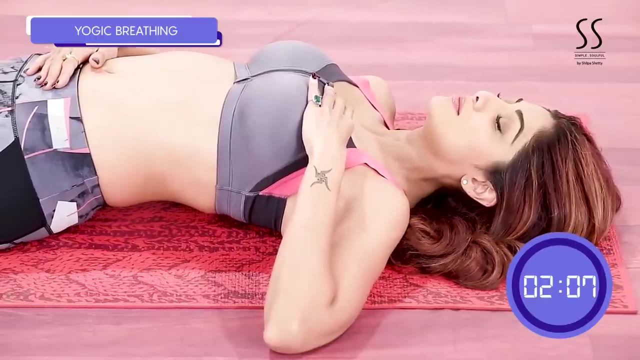 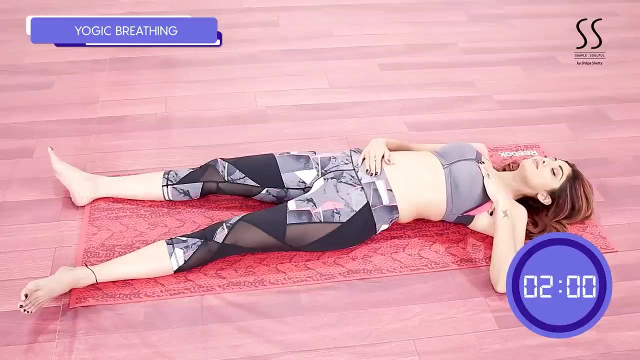 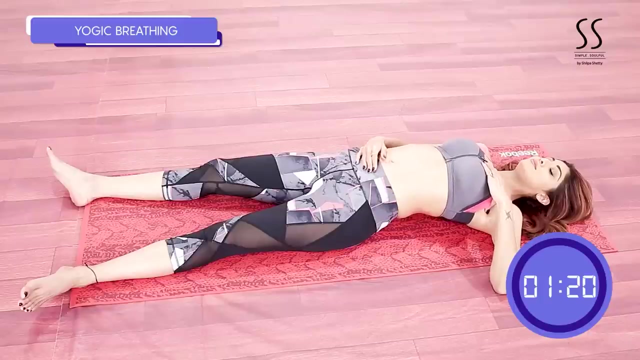 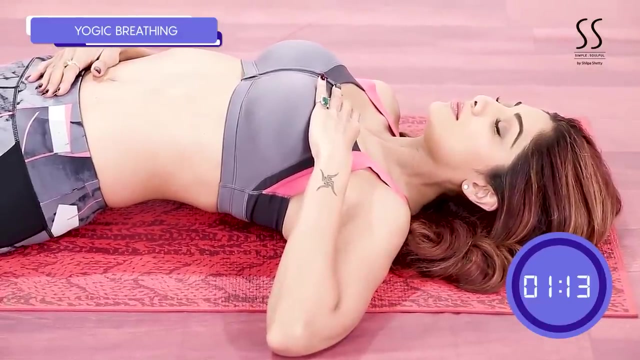 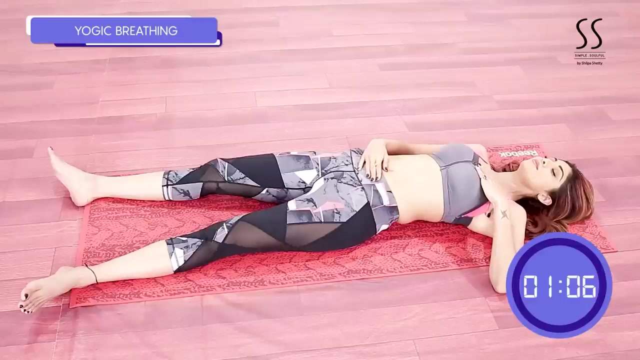 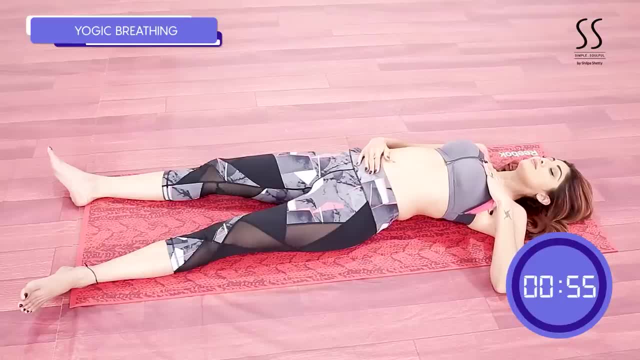 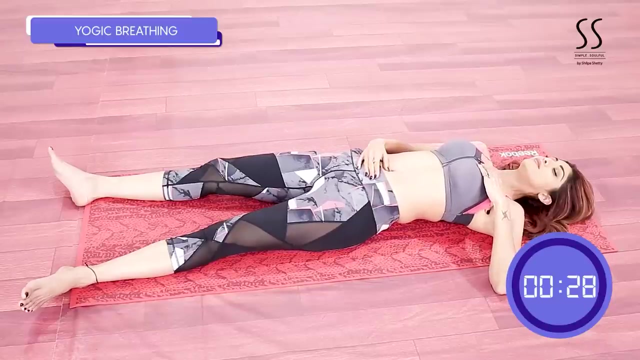 When the belly is full, draw in a little more breath and let that air expand into the ribcage. Let it fill the upper chest all the way up to the collarbone. Feel the body relax with every exhalation. There should be no tension on the face or arms. 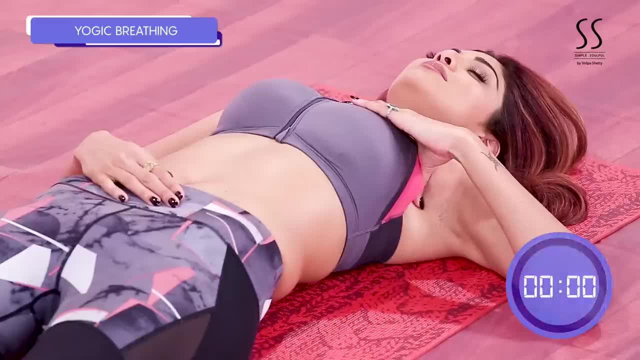 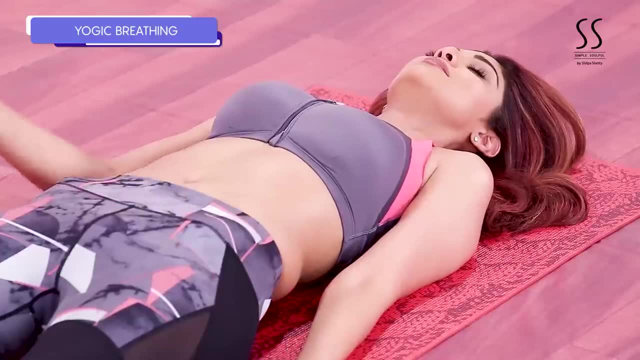 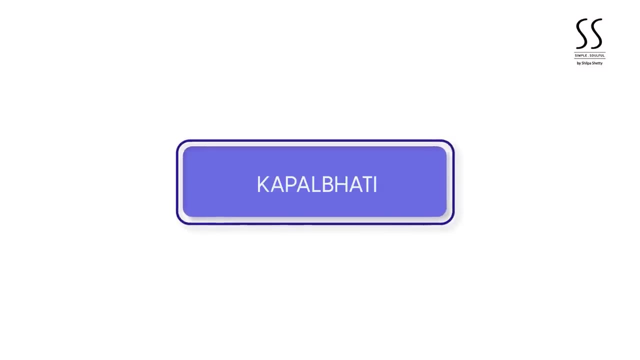 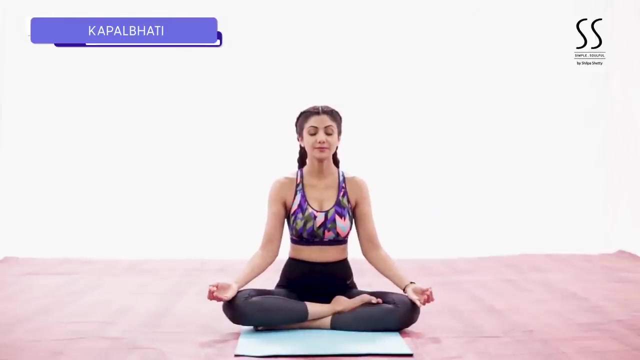 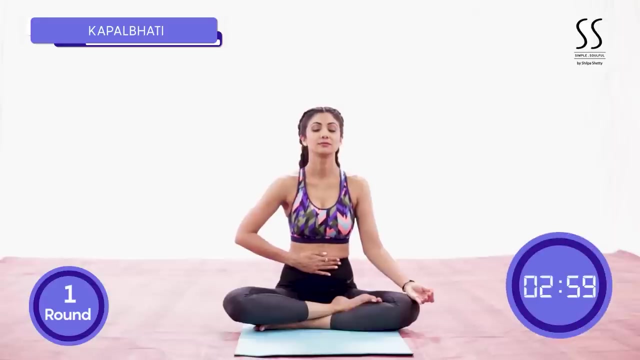 Feel the body relax with every exhalation. Deflate on exhalation. Keep your right hand on your abdomen to observe the breath. Take a deep breath with both your nostrils, Exhale forcefully through both your nostrils and keep deep contraction in the abdomen. 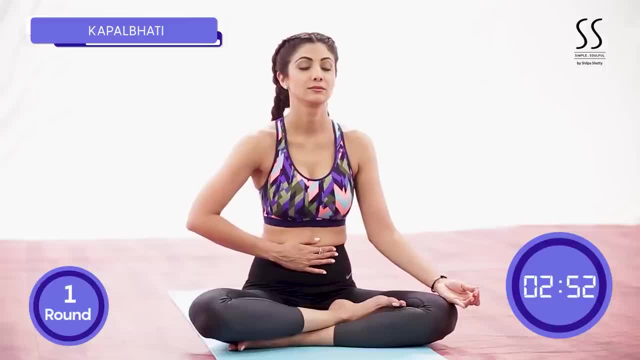 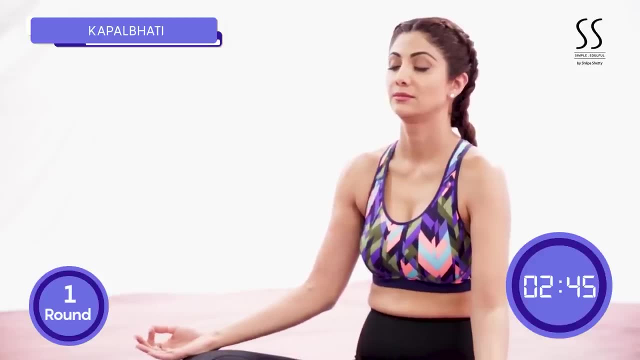 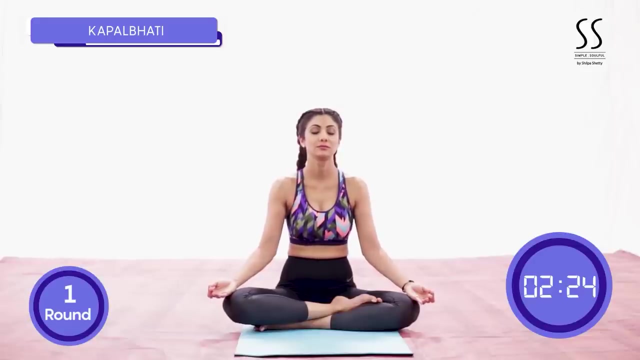 Inhalations are shallow and quick, whereas the exhalations are forceful. Relax your shoulders and chest. It is important that the rapid breathing should be from your abdomen and not from your chest. Maintain tall posture from the lower back to the neck in the entire spine. 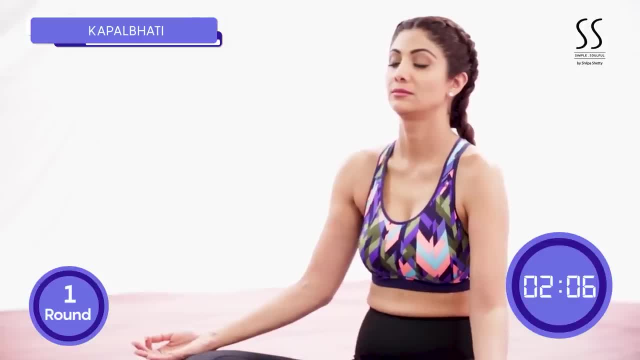 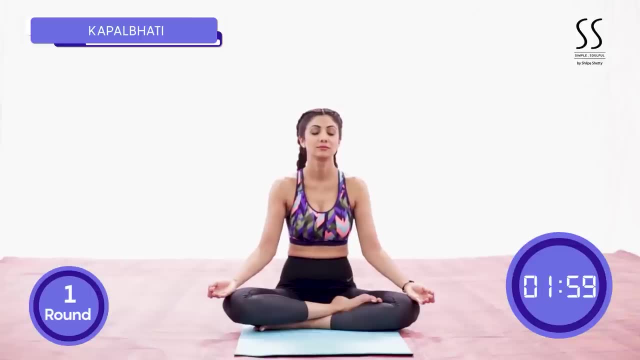 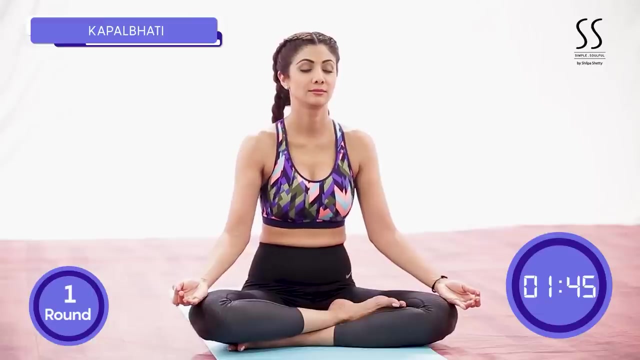 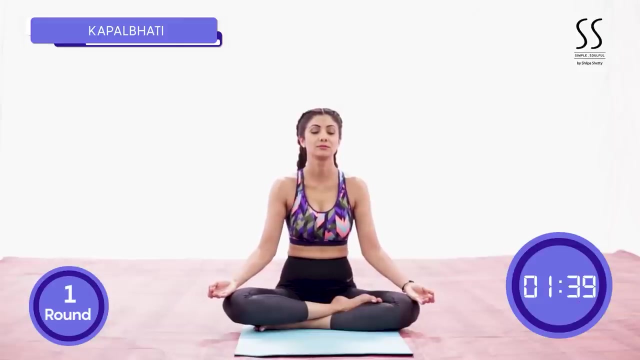 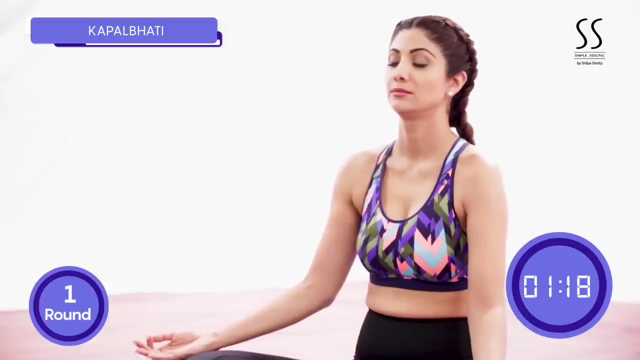 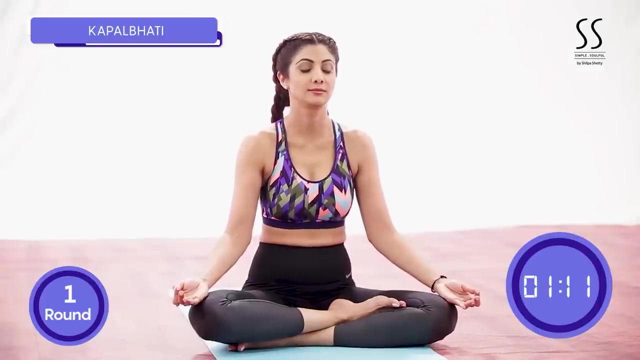 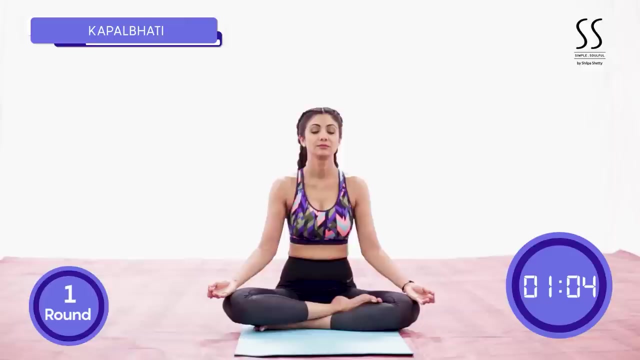 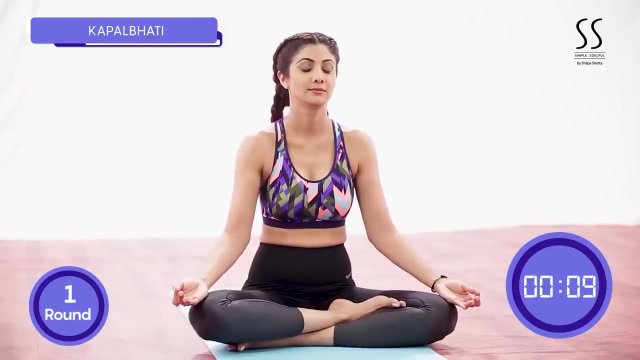 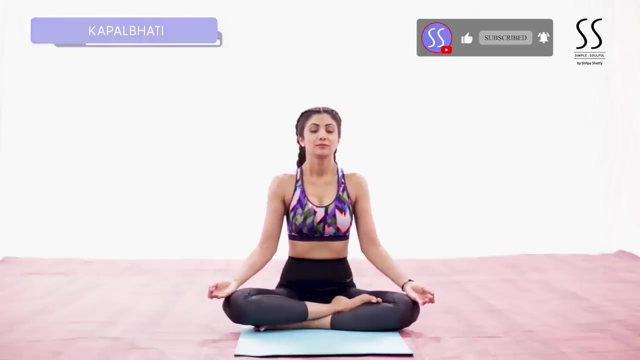 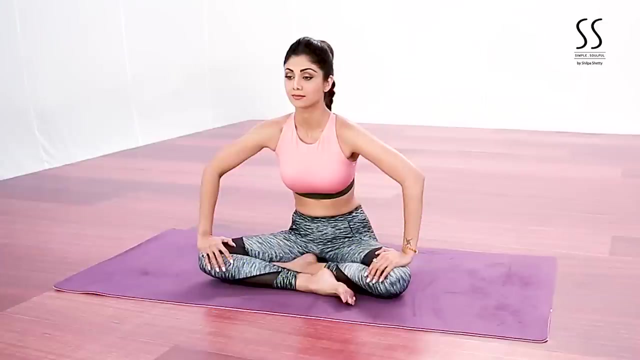 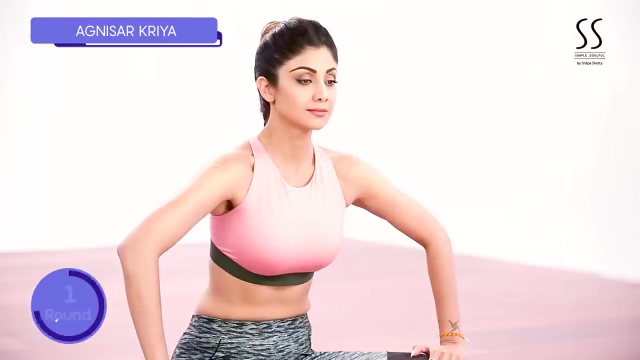 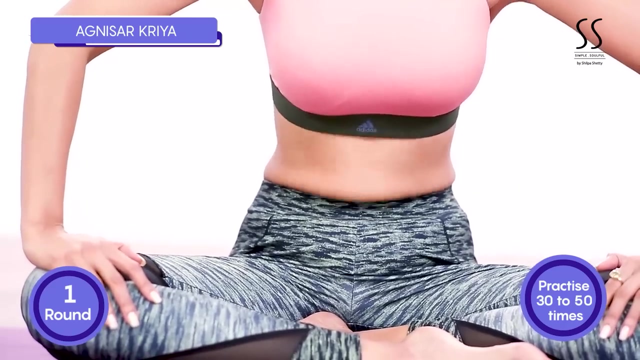